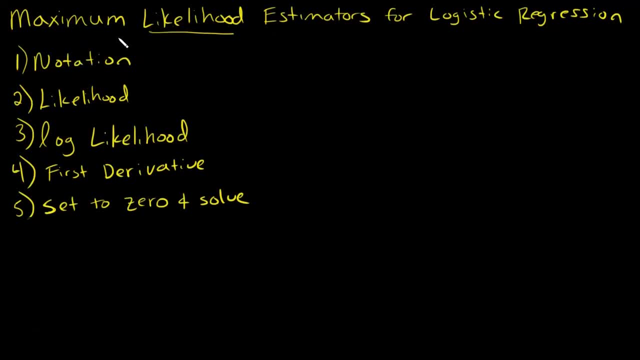 Okay, so let's start with the notation. all right, so let us assume that yi follows a Bernoulli distribution. Now, why Bernoulli? Bernoulli? because Bernoulli is a distribution for zeros and ones. all right, so follows a Bernoulli. 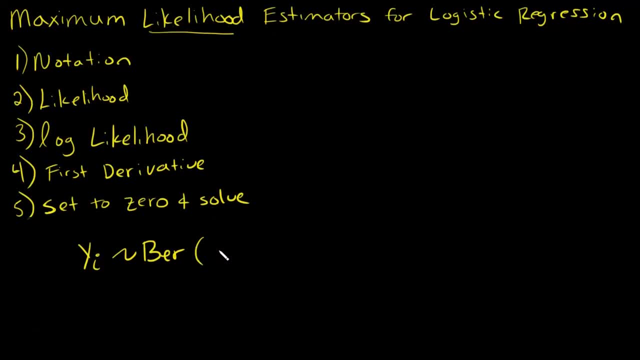 distribution and the probability that y equals one right, which is the parameter that a Bernoulli distribution takes, is going to be pi and I'm going to take all of those independent variables, xi. all right, so xi is going to be a. 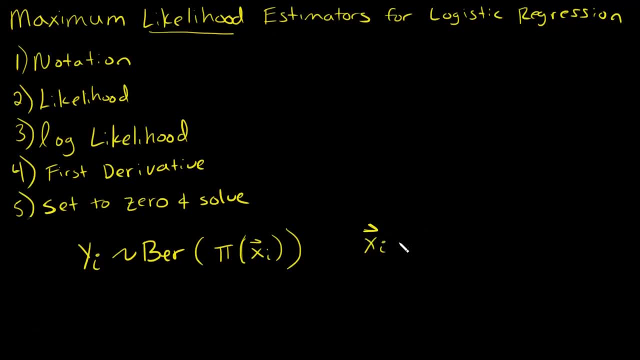 vector. so to note that it is a vector, I give it this little hat and it's one. okay, one, i, two, i and then say I have p independent variables. okay, and the reason why there's this one, this first leading one, is for: 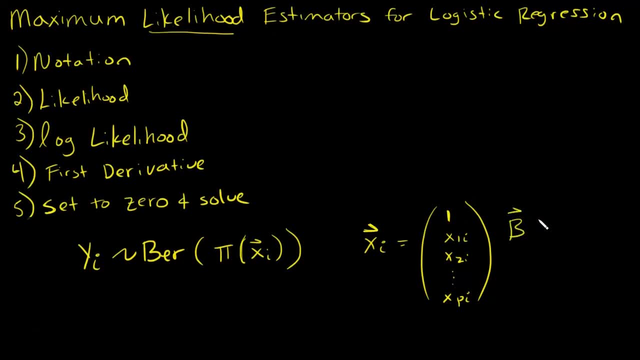 an intercept. all right, I'm going to go ahead and define my coefficients, beta, right, these are what I want to estimate. beta is beta naught, which is the intercept beta one, all the way through to beta p. all right, so yi is going to be a vector and I'm going to take all of those. 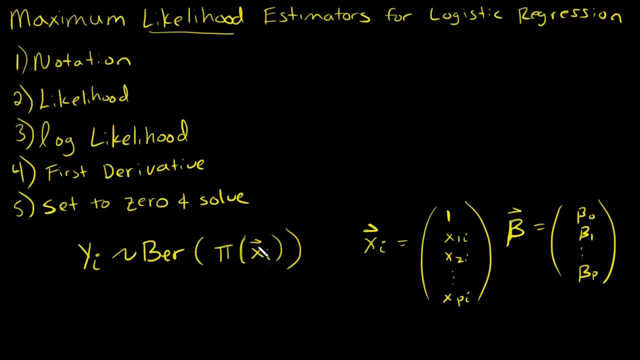 independent variables. okay, so I've got my negative xi transpose times beta. okay, And this comes from the logic function, all right, Which I think that that is worthy of a video of itself. okay, So I will include another video where I'm going to discuss this logic function. 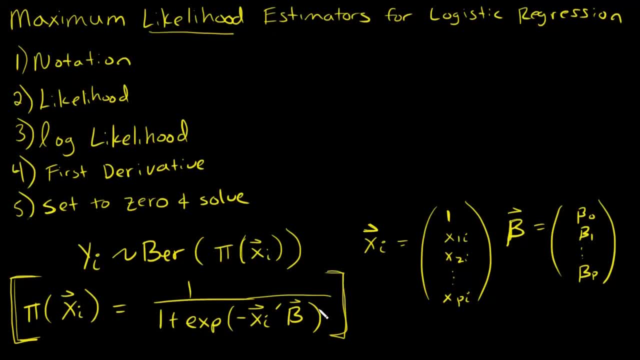 But basically you can find this relationship with the logic function, which is the probability that y equals 1, equals the log of the probability that y equals 1 divided by the probability that y equals 0,. okay, This is the logic function. 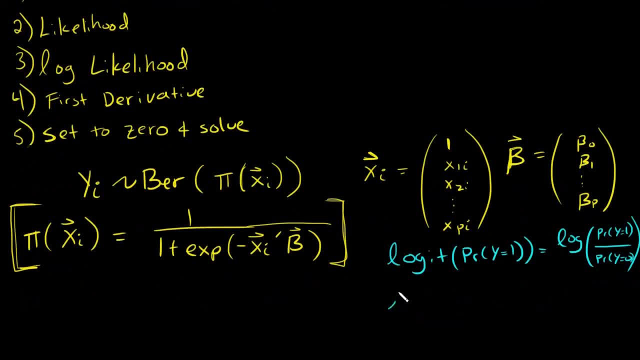 And in logistic regression the logic function probability y equals 1, equals x, transpose beta. okay, So this is this linear term here that is equal to the logic function. all right, So if you were to rearrange this, you could find what we see here. 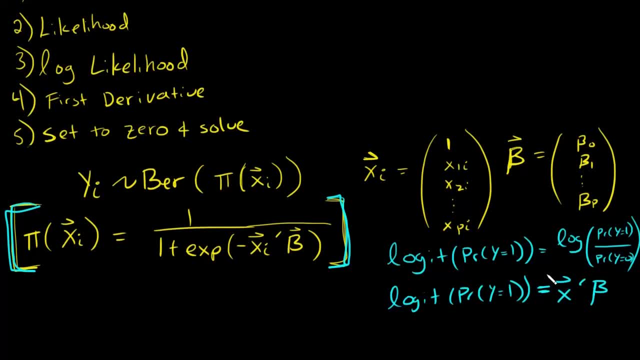 And, as I said, I can show that in another video. but it kind of takes a little bit of time to build up between those two. But you could spend, you know, a few moments and try to rearrange this and show this relationship. 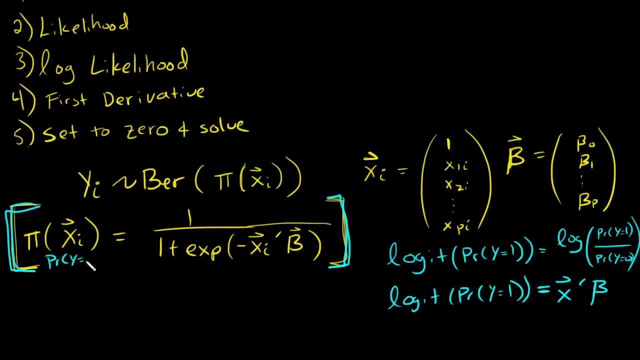 Because remember what is pi of xi. This is equal to the probability that y equals 1, right By definition of the Bernoulli. Okay, so setting up notation still, so that I do not have to. I can kind of be a little bit lazy. 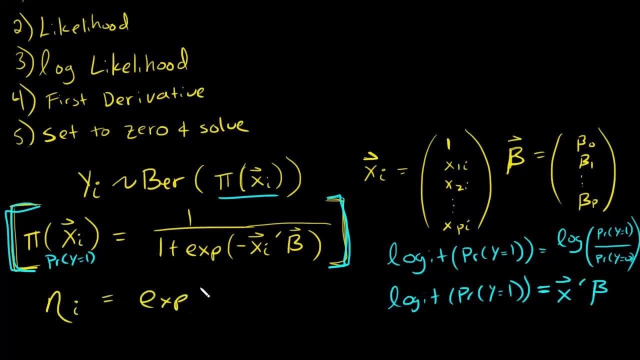 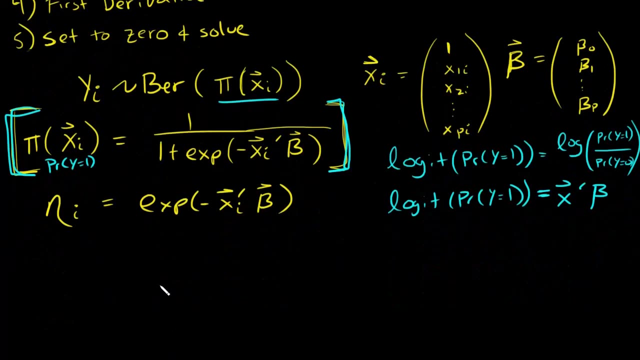 and I don't have to write exp, negative, x, transpose, xi, transpose times, beta So many times. Instead, I'm just going to call that nu i right, And that's just for convenience as I'm doing this derivation. All right, so now I have. 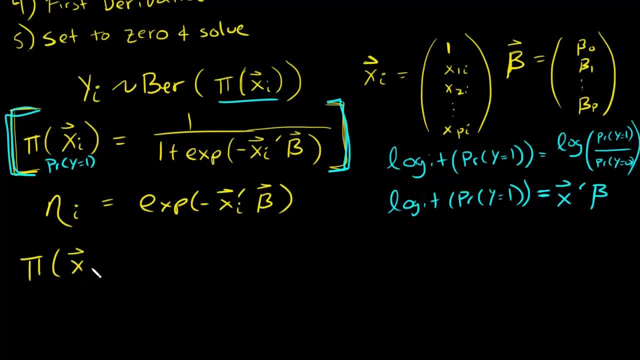 the probability that y equals 1, or pi of xi, This equals 1 over 1 plus nu. i. all right, All right, so that's my notation. So this is number one, all of my notation. Okay, So now? 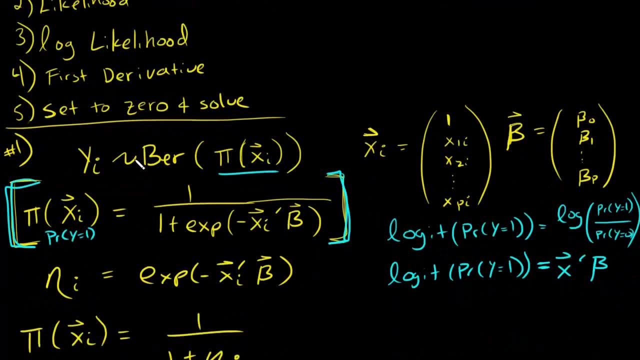 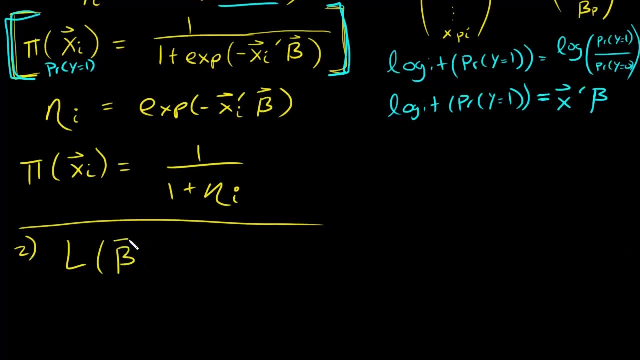 let us do number two, which is define our likelihood function. All right, So likelihood function with regards to these coefficients, beta. All right, In general, that this is the well. actually let me skip ahead. In general, a likelihood function. 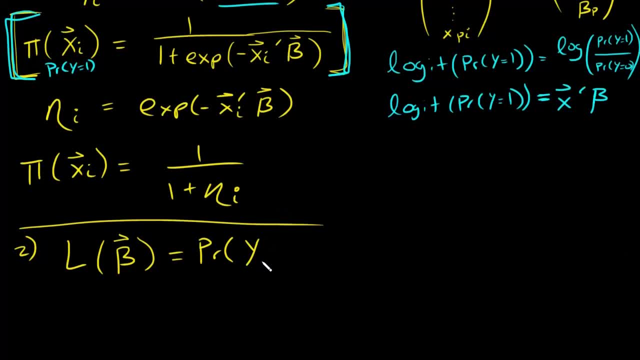 is the probability of basically all those different y's that you have. Okay, That's what a likelihood function is, All right. And since we're assuming that all of our y's are independent, right, we can say this is the probability. 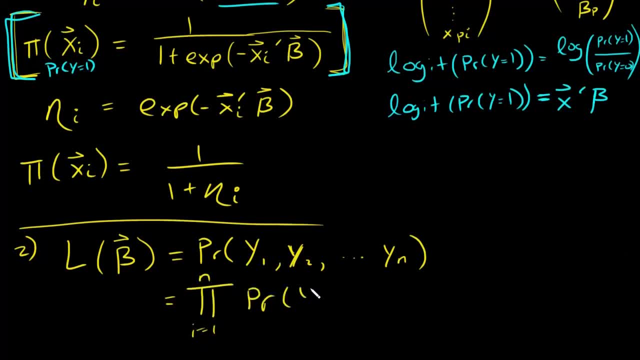 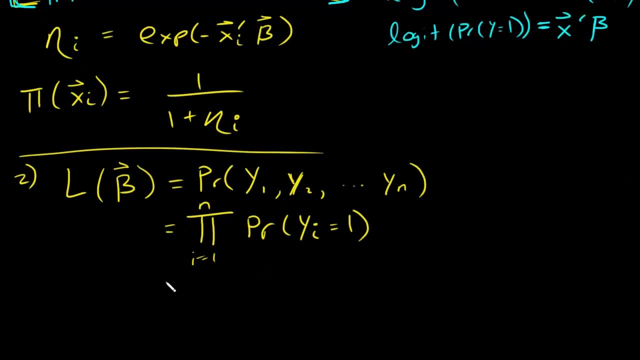 the product of all the probabilities. Okay, y i equals 1.. Okay, So the product of all the different probabilities. Well, we have a Bernoulli distribution for the probability of y. Okay, So what is a Bernoulli? 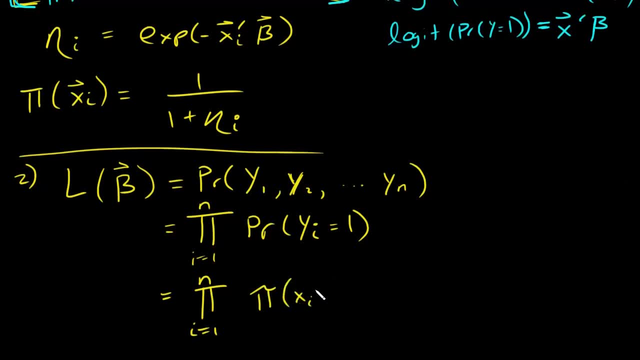 It's going to be this: the probability that y equals 1, which is this pi of x? i to the power of y i, 1 minus pi of x? i, and then 1 minus y i. Right, This is straight up what the Bernoulli distribution. 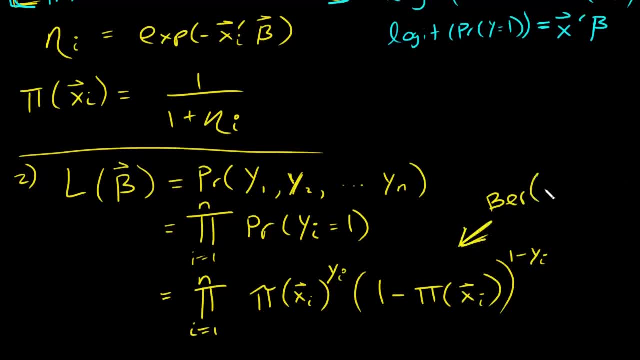 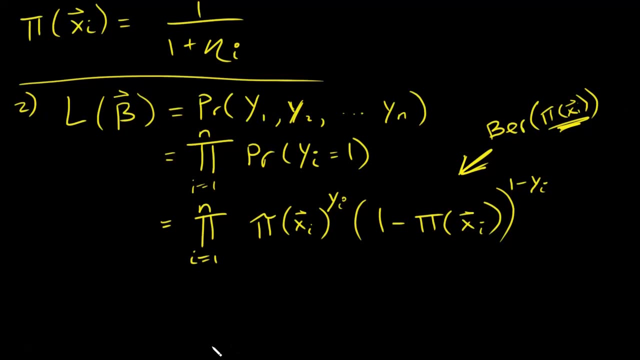 looks like: Okay, A Bernoulli with parameter pi of x i. Okay, So instead of it just being p, now it's pi of x i. All right, Okay, So we can do some simplification. So before moving on, 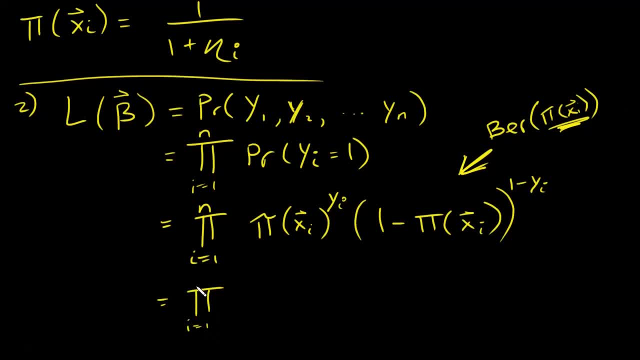 let's go ahead and plug in: what is pi of x i? Okay, So the product from i equals 1 to n. All right, What is pi of x i? It is 1 over 1 plus nu i. Okay, 1 over 1 plus nu i. 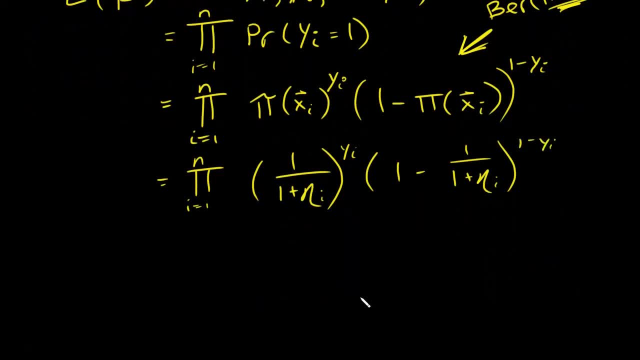 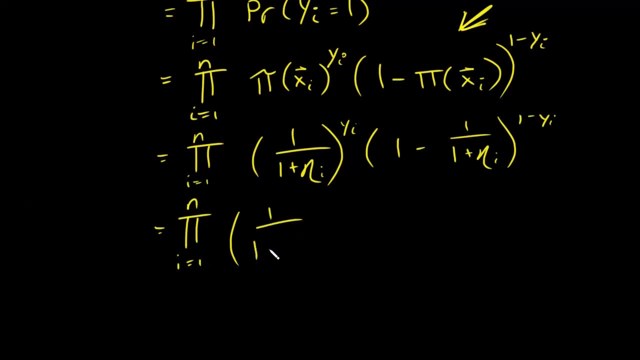 All right, So let's do some more simplification. All right, So let's simplify what we have over here. All right, So 1, right. if I want to simplify this, this is: the 1 is the same thing as 1 plus nu i. 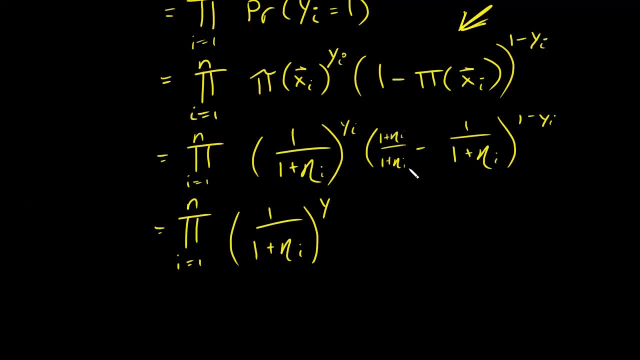 over 1 plus nu i, Right? Why did I do that? Because I want the same denominator, So now I need to subtract this. Okay, So the 1s will cancel and I'll be left with nu i in the numerator. 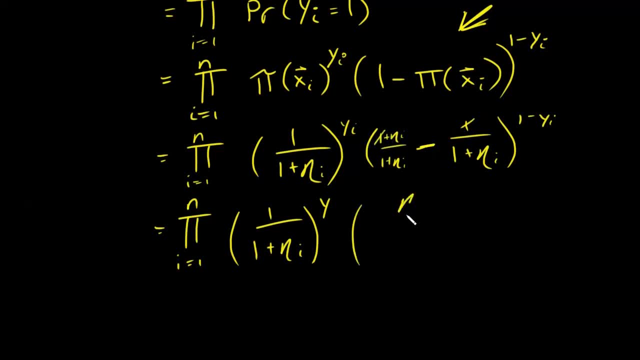 and then 1 plus nu i in the denominator. All right, All right, That's as simple as I'm going to get for the likelihood function. Okay, So beta is a vector, so that's why I have the little hat. All right. 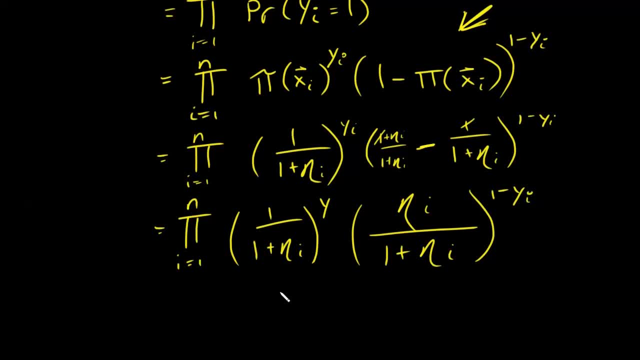 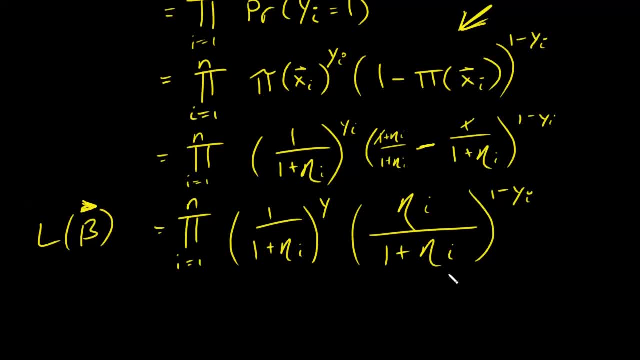 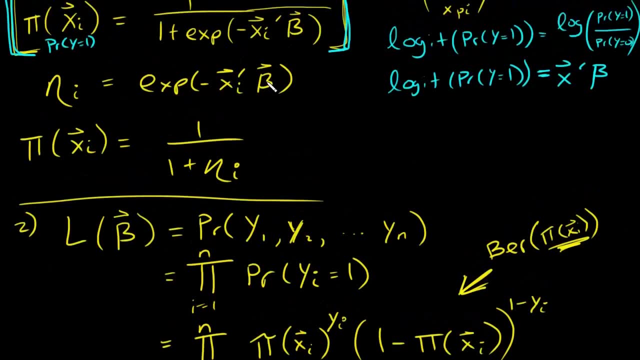 over 1 plus nu i over 1 plus nu i over 1 plus nu i. all right, And remember, beta is sitting inside these nu i's right, because what is nu i There, it is, It has that beta Okay. 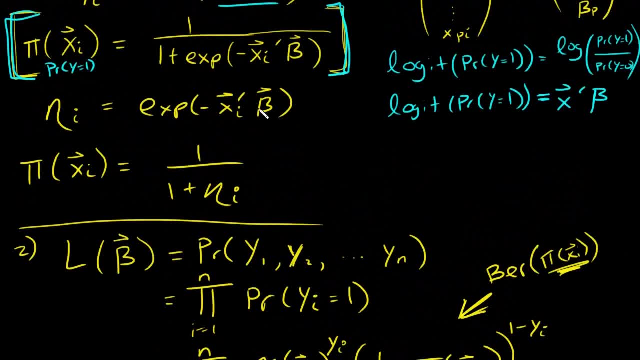 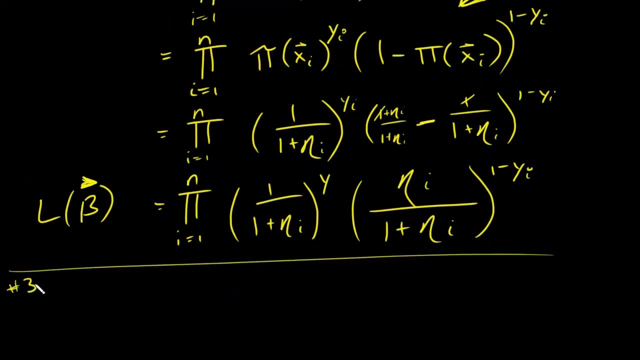 So it's a little confusing because you don't see any betas over here, but they're inside that. nu, i All right. So that's my likelihood function. So now I'm ready to find my log likelihood. Again, we do log likelihood. 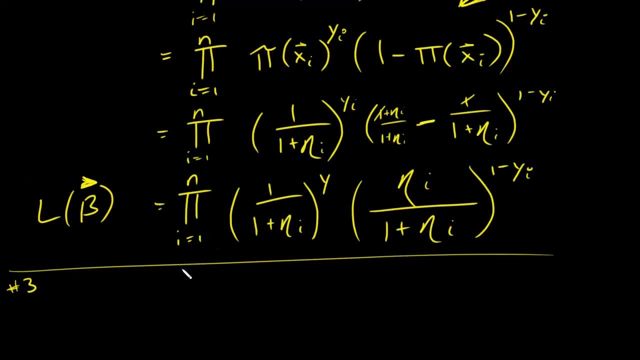 because when I'm taking a derivative, it's a lot easier to find the derivative of a bunch of sums than the derivative of a product. And and since the maximum of the log function is the same as the maximum of the function, you know. 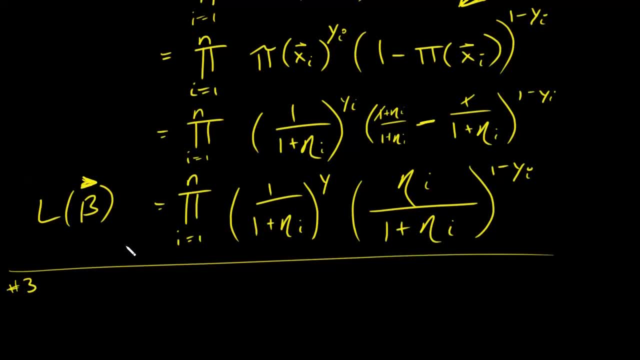 it's a nice, it's a nice property. It's helpful for us to use log likelihood when we're looking for a maximum likelihood estimator. Okay, So log likelihood, All right. So when you take the log of this, all of these, 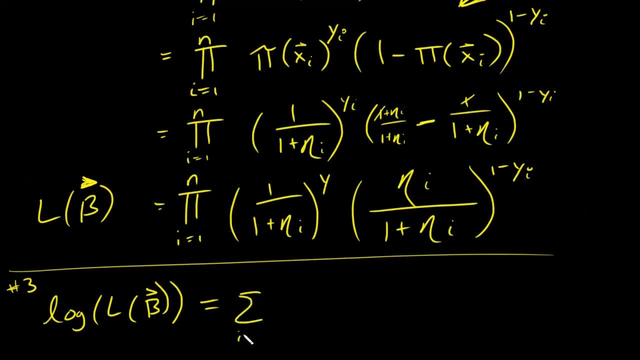 the products. the products become a sum from i equals one to n. Okay, Then I'm going to have the ln one plus nu. i to the y. i Looks like I dropped my i there. All right, So then this: this is a product here. 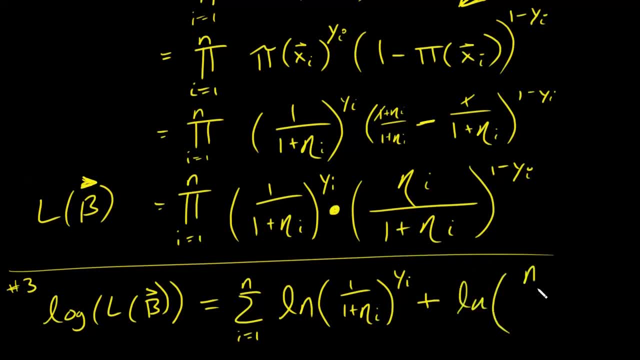 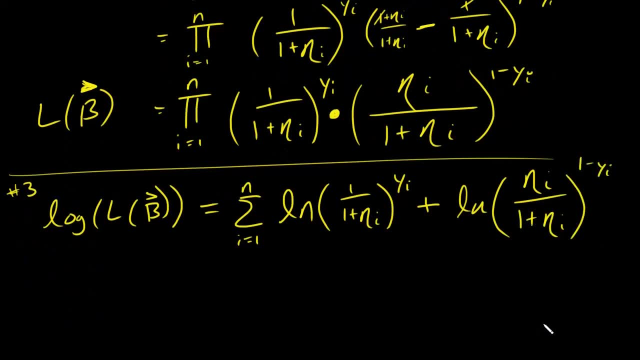 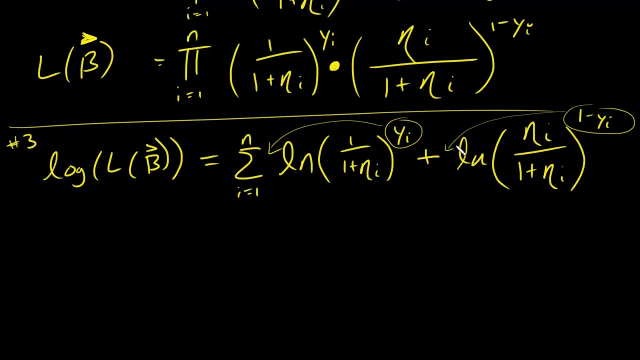 So that becomes a plus right, The ln of nu i, one plus nu i. All right, Let's do some properties of log. Okay, So we can take this exponent and bring it down, All right, So I end up with the sum. 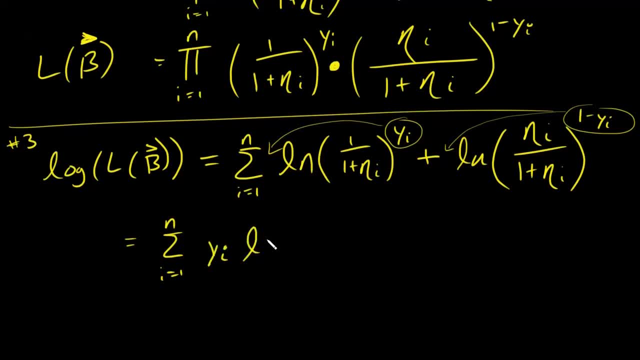 from i equals one to n of y, i ln of one plus one plus nu i plus one minus y. i times the ln of nu i one plus nu i. Okay, So now I can do some more simplification, right? What is this? 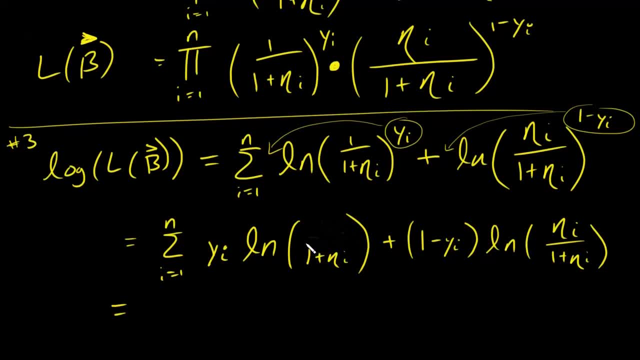 This is the same thing. So it's one over. So that's the same thing as to the negative one power. So now, once again, I can bring that down, And so I have the sum from: i equals one to n of negative y, i. 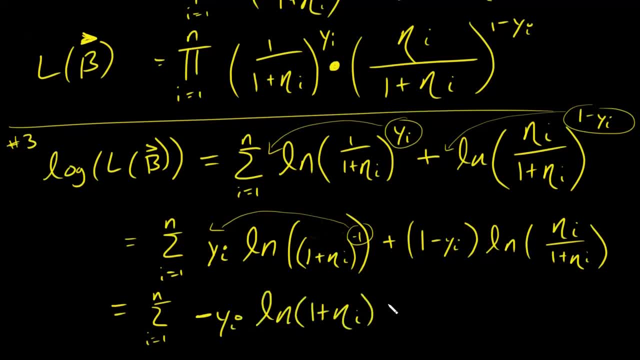 the ln of one plus nu, i Okay. Plus one minus um, um, y, i All right. And then I can do a similar. So I have a you know division here. So this is the ln of uh. 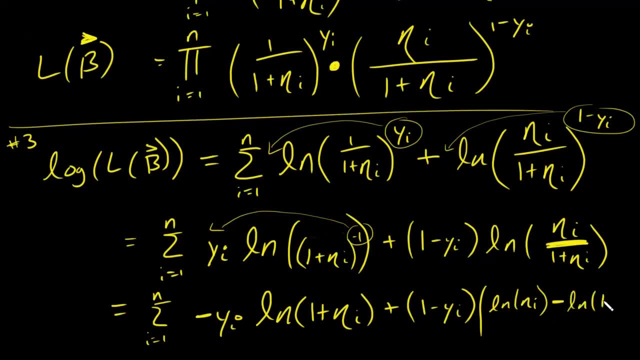 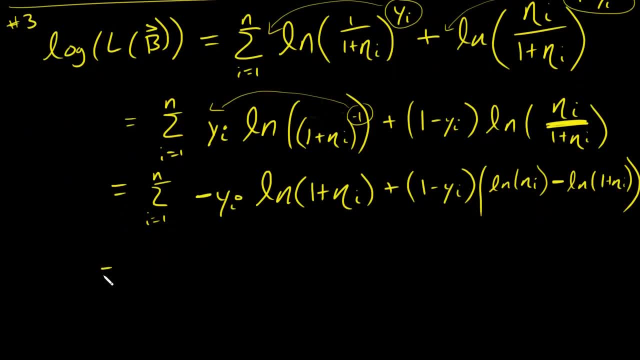 nu i minus the ln of one plus nu i. All right, So I'm just kind of using some properties of log. Okay, We can still simplify this some more. Okay, I'm just rewriting that first part. Okay, Now over here. 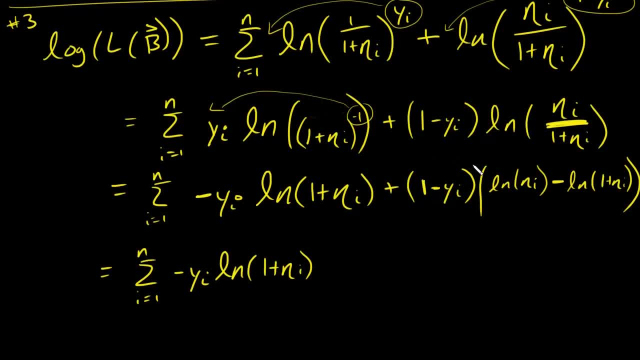 I have basically two binomials. I can just FOIL them Right, Multiply by the first and then multiply by the second. So what do I have? I have, um, the ln of nu i minus the ln of one plus nu i. 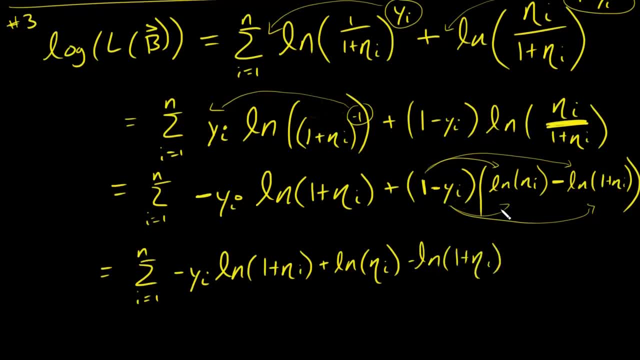 Then I have minus y i times the ln of nu i- Okay. And then I have minus y i minus the ln of one plus nu i- Okay. So let's see if I have any cancellation, And I do. It looks like this guy. 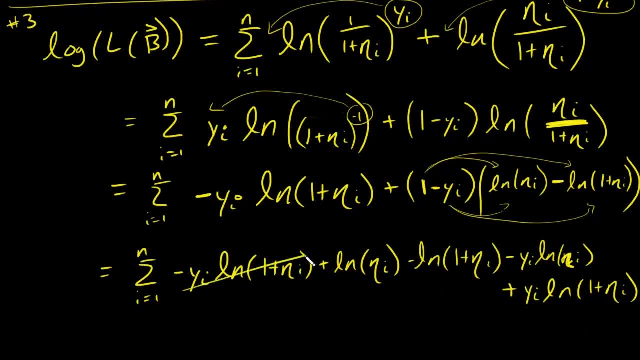 cancels with that guy, All right, And I think that that is the only cancellation that I have. All right, Let me just double check. Yep. So then this: u is minus the ln of one, plus nu i, Yep. So then. 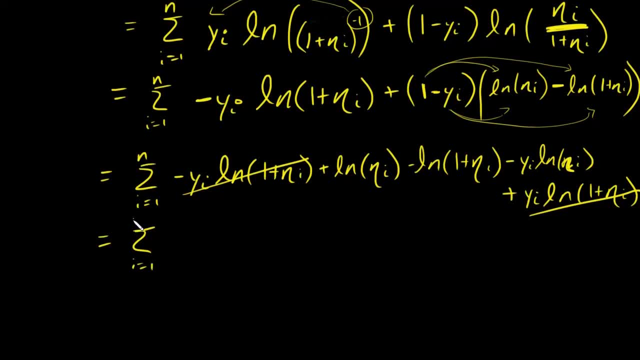 this equals the sum from: i equals one to n. And what do I have? The ln of nu i minus the ln of nu i minus the ln. actually, um, let me take that y out, All right, So I have um. 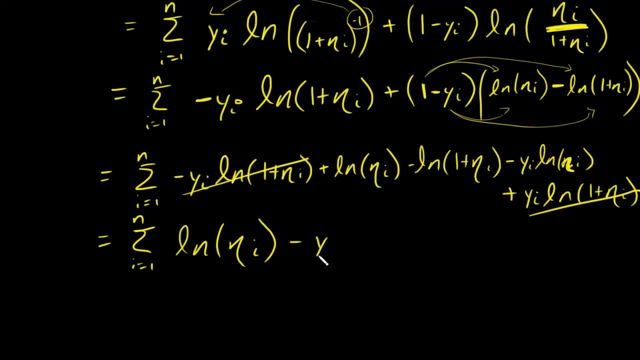 let's see: um y i, nu i- Okay. Then minus the ln of one, plus nu i- Okay. So I wanted to write these guys next to each other because they have like terms, Okay. So now I can actually simplify this a little bit. 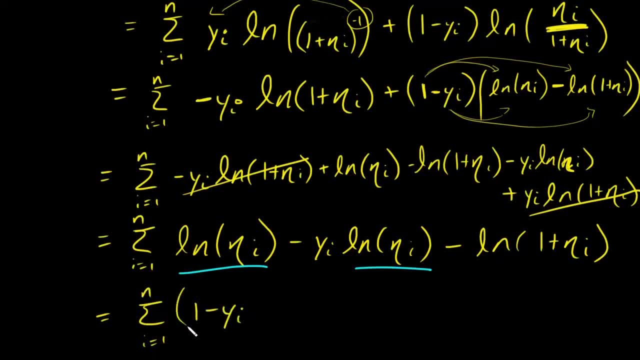 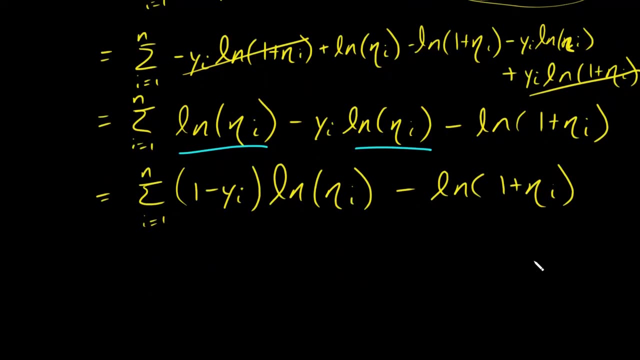 more. And what do I have? I have one minus y i times the ln of nu i minus the ln of nu i. Okay, Great. So this is my log likelihood function, And I'm going to need to take the derivative here in a second. 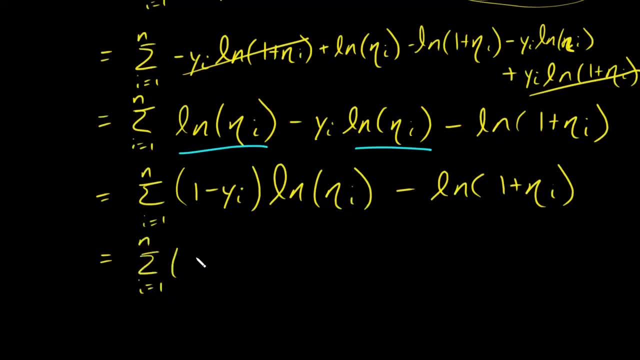 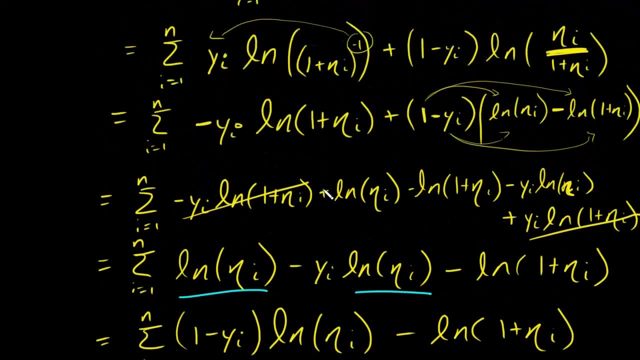 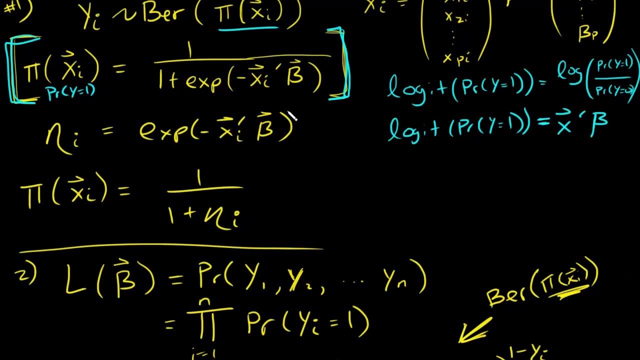 So let's go ahead and plug in for nu i. What is nu i? It's the ln of. okay, let's scroll back up to look at what is nu i. e to the power um x. i transpose times beta. Okay. 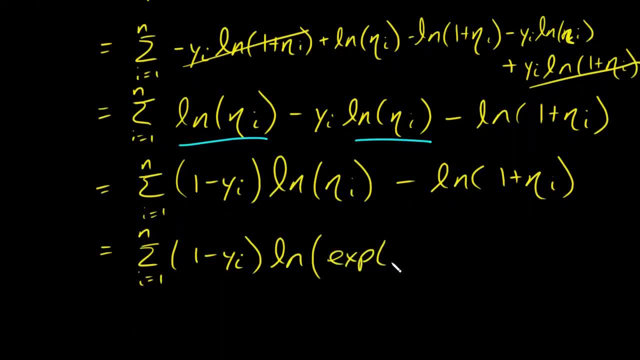 So what is this? Um? e to the negative x transpose times beta. Okay, So I just plugged in for nu i there, Minus I'm going to run out of room, so I'm going to do this down here, Minus. 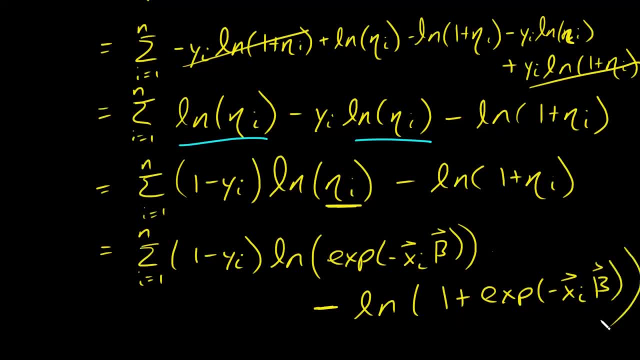 1 plus e to the power of negative x. i transpose times beta. So let's see, here I have. um, this guy will cancel with this guy, right? So I have. this is equal to. i equals 1 to n of. 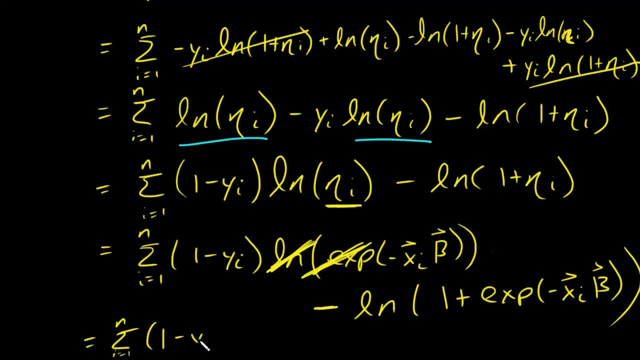 1 minus 1 minus y i. And then I have this multiplied by negative x, i times beta x. i transpose times beta should be transpose there. Okay, Minus this ln of 1 plus e to the power of negative x, i transpose times beta. 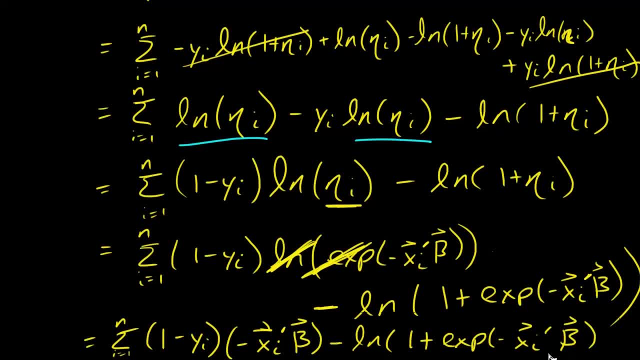 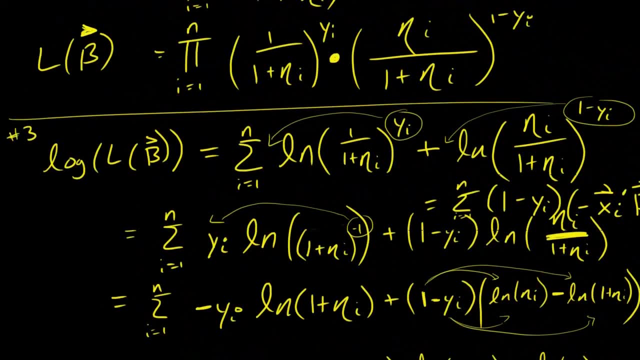 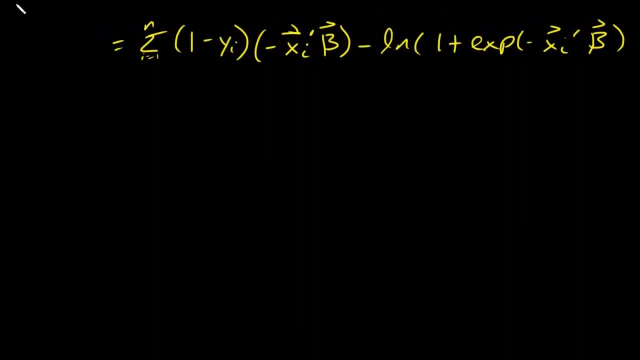 Okay, So now I've run out of room on my screen, so I'm going to um move this up. Okay. So this is the uh log likelihood function, right, which is the end of step three. All right, 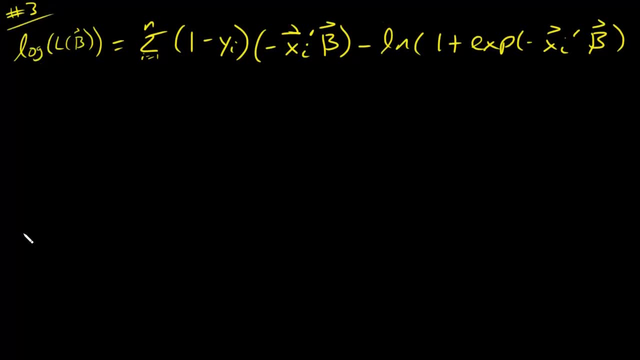 So once we have the log likelihood function and we're trying to find the maximum likelihood estimators for beta, the next step will be to find beta. So let's go ahead and do that. Uh, what we want to do is: 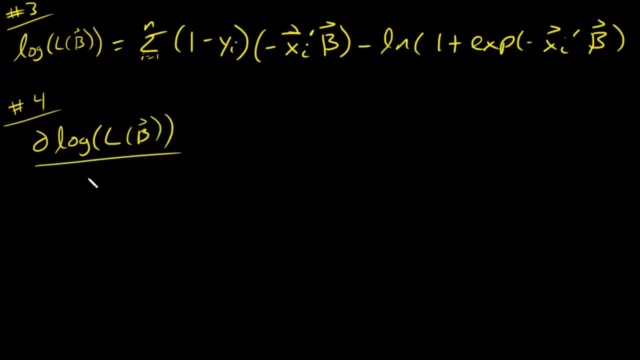 find the derivative of the log likelihood function with respect to beta. Okay, So we have: the sum from i equals 1 to n. Okay, And so now, when I take the derivative of this piece here right, I will have 1 minus. 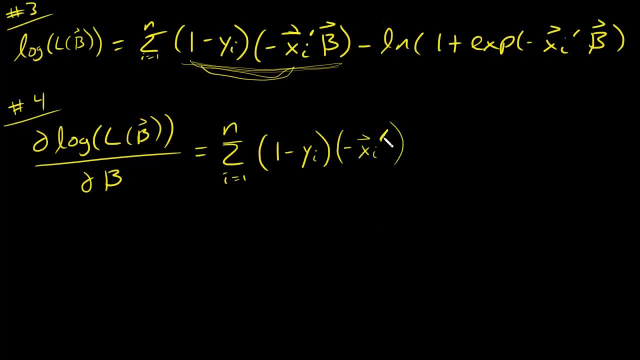 yi times negative xi transpose: All right, I'm taking the derivative with respect to a vector. All right, So I'm taking the derivative with respect to this vector here. All right Now. so that would be 1 over what's inside. 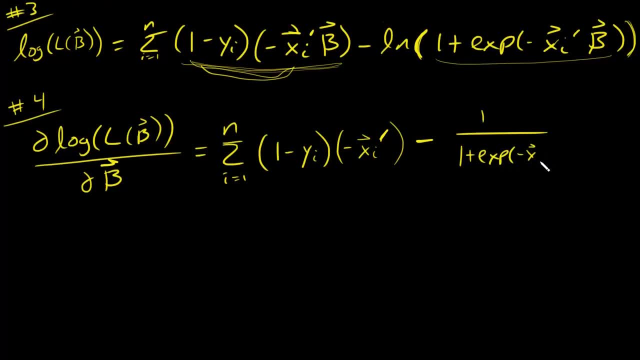 of the log. Okay, So this is going to be quite a bit of a chain rule here, Okay, And then I take the derivative of what's on the inside of the log right, which would be the derivative of the inside of the. 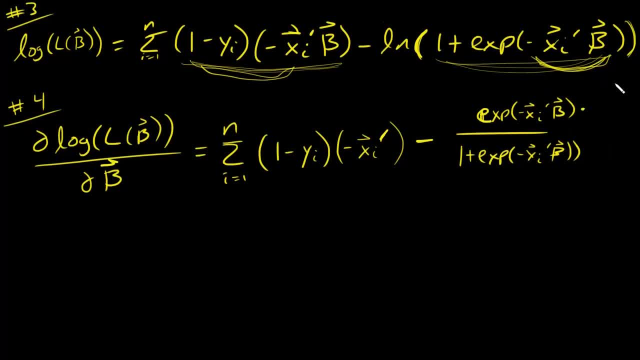 e, so the exponential power, right. So this would be multiplied by the inside of this would be just negative xi transpose. Okay, All right, Good, So let's see here. So I can pull that negative sign out and I have 1. 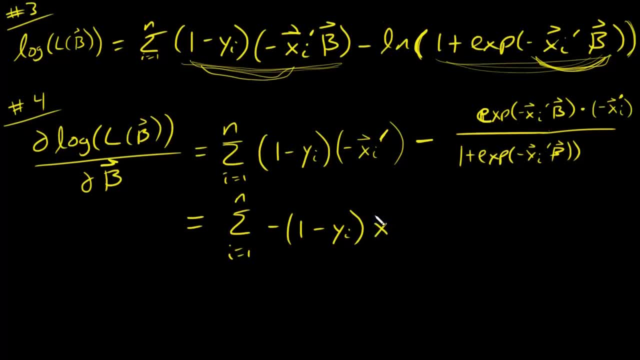 minus yi times xi transpose Okay. Minus plus, because the minus and the minus here make a plus. e to the power of negative. xi transpose times beta: All right. Times xi transpose Okay. So lastly, you could pull out. 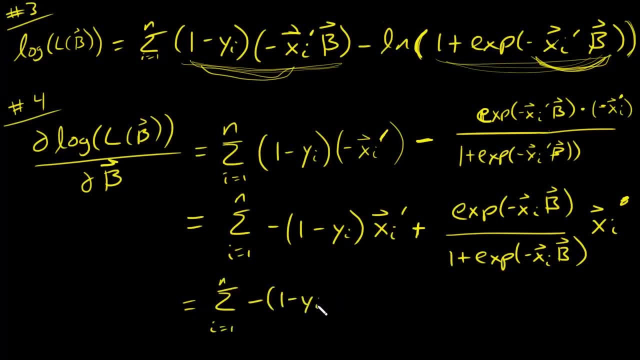 So we'd have negative 1 minus xi or yi All right, Plus e to the power of negative times beta 1 plus e to the power of negative xi transpose- I forgot my transpose Times beta Right. Note that this piece here: 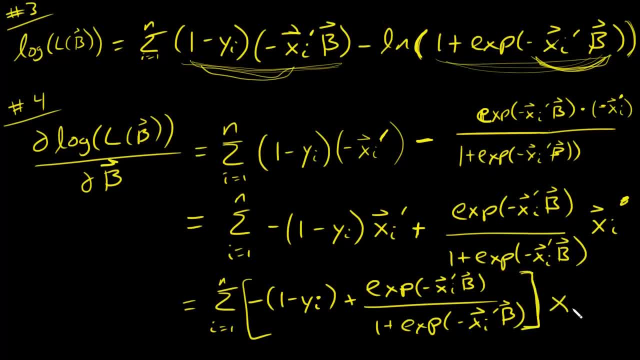 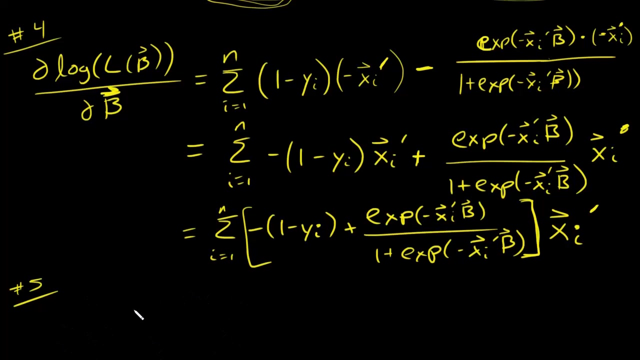 is a scalar, All right. And so then it gets multiplied by xi trans this vector here. So it's 1 minus yi plus e to the power of negative xi transpose, All right. So that's why this: I'm taking the derivative with: